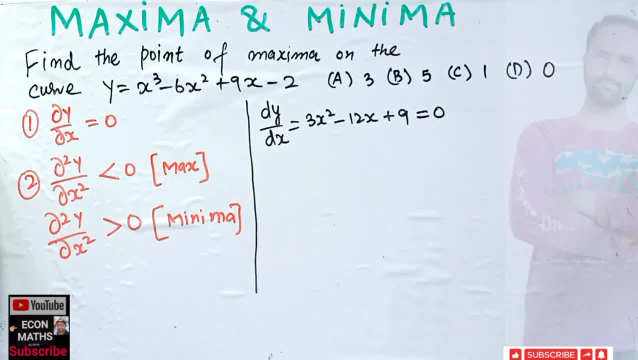 Okay, Now let us solve this very question. Quadratic equation to say so. So we have 3x square minus 12x plus 9.. Let us take 3 common. Okay, We can write it like this: x square minus 4x plus 3 is equal to 0. If I transpose this, it will become 0. So this 3 gets cancelled or it vanishes here. So we have: x square minus 4x plus 3 is equal to 0.. So just splitting the terms you know, So we will get x square. 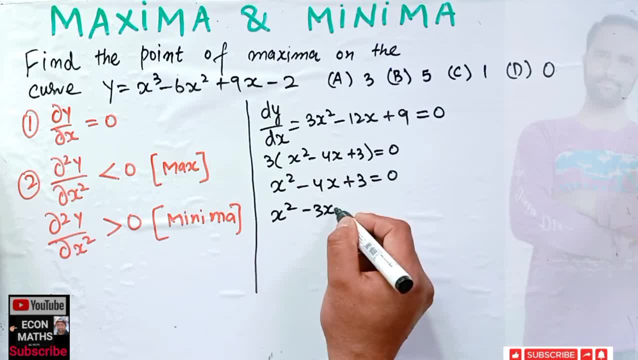 We have minus 3x. We have again minus x. plus minus 3 into minus 1 is equal to 0. Okay, Taking common factors here I have just splitted the middle term here. Okay, So sum of the numbers should be minus 4 and the product of that same number should be 3.. So we have minus 3 and minus 1 comes out to be minus 4, and minus 3 into minus 1 comes out to be plus 3.. Okay, So, taking factors common, We have: 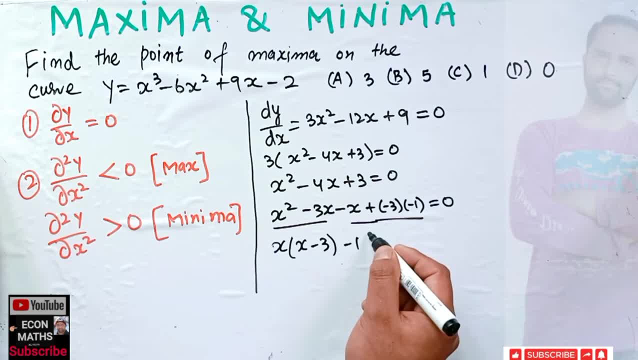 x here, so we get x minus 3. taking minus 1 here common, so we are left with x minus 3 again. okay, if i take minus 1 here common, so we will get x minus 3 and we set it equal to 0 here. okay, so this means either x minus 3 or x minus 1 is equal to 0. that means we got two values. 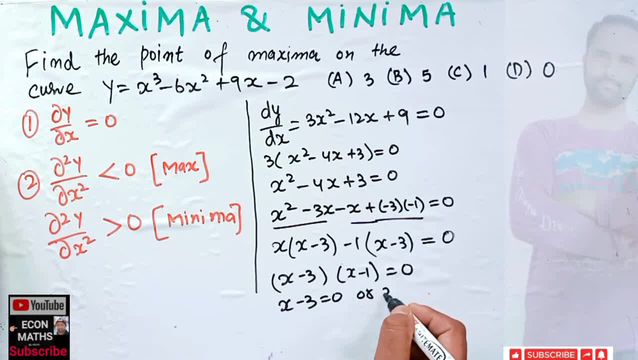 x minus 3 is equal to 0, or x minus 1 is equal to 0. that gives us x is equal to transposing. it can gives us 3 as the value of x or x. if i transpose this minus 1, so this will become 1. okay, so we got. 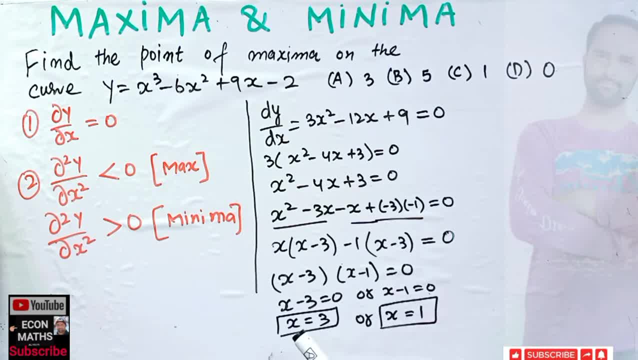 two critical points. now we have to see which of these two pointers is maxima or minima. so this was the first condition. we set the first derivative of our curve with respect to x equal to 0, and we got two points, that is, x is equal to 3 and x is equal to 1. 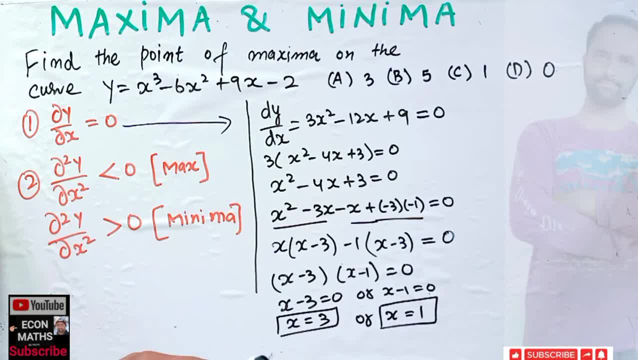 now we have to see which of these two points is maximum in fact. okay, so for that we need to check the second order condition. okay. so second order condition is simply, we take the second derivative d square, y upon d x square, and evaluate at critical points. first we evaluate it at 3 and 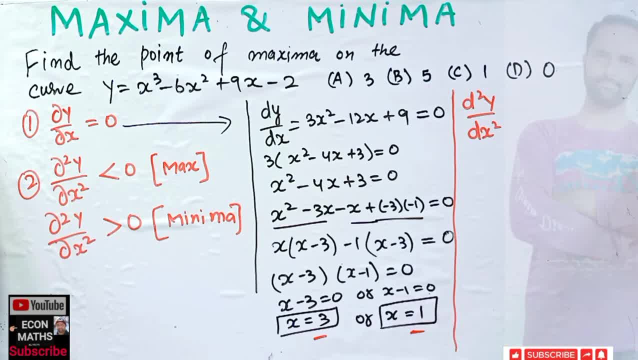 then evaluate the second derivative at 3, and then evaluate the second derivative at 3, and then evaluate it at 1 and see what will be the sign of the second derivative. okay, so let us write it like this: if i evaluate it at, x is equal to 3. okay, so first let's take the second derivative. this is: 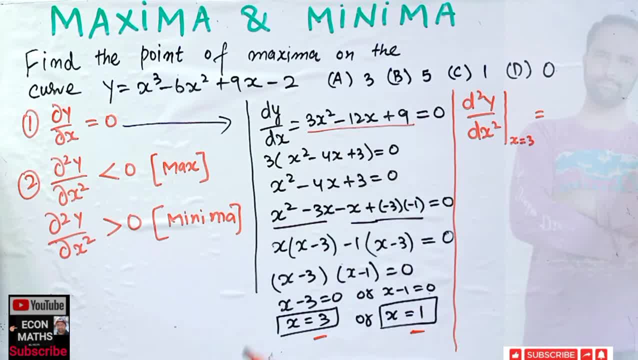 first derivative. so second derivative is the derivative of this function, again with respect to x. so we have two. threes are secs. secs x, derivative of x is 1, so we are left with minus 12. okay, if we evaluate it at, x is equal to 3, so we will get 6 into 3 minus 12, so this comes out to: 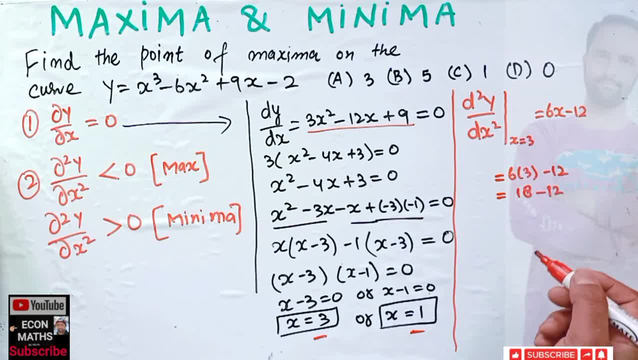 be 18 minus 12. okay, so this comes out to be ardhanibhata shares, but this is greater than 0. okay, so this point x is equal to 3- will be for minima. okay why? because if the second derivative comes out to be greater than 0, then we: 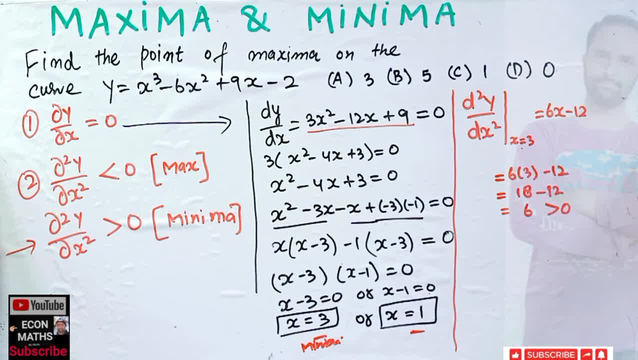 have case of what we are what we call minima. okay, so let's check it at when x is equal to 1. okay, so we have d square, y upon d x square, and let us evaluate it at x is equal to 1. so what will we get? so this is our second derivative: just plug this critical value here, so we have. 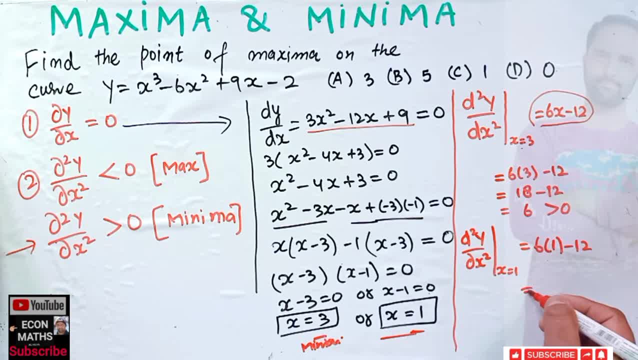 6 into 1 minus 12, which comes out to be 6 minus 12. so we get this, which in fact is less than 0. okay, so for the maxima, two conditions were required: first, that we set the first derivative equal to 0, and second, derivative should be less than 0, and here: 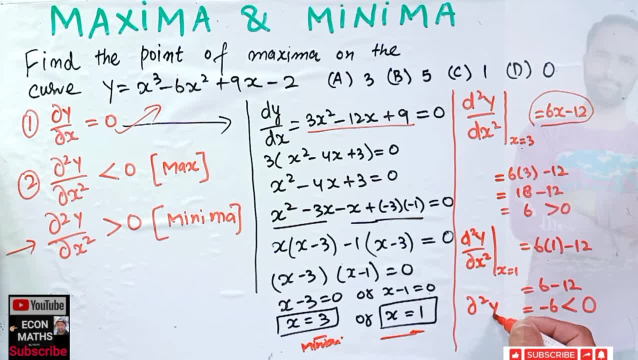 we can see. second derivative, in fact, is less than 0, so we can safely say that the point of maxima will be 1. okay, and graphically, what does this mean? it is simply, if we have, let us try to draw the graph. i will not be able to show it perfectly, but let's try to draw. 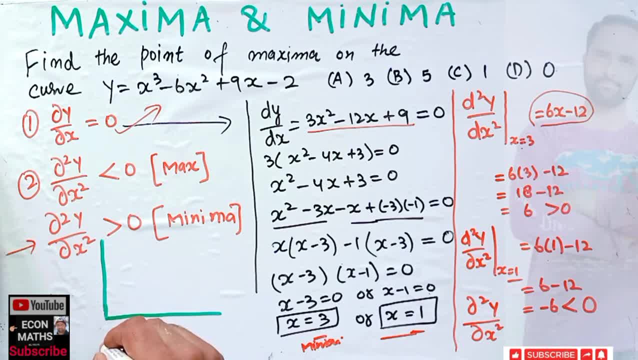 so our function would have been like this: okay, so we got two points. okay, this is our curve, and we were told to find the maxima on this point. okay, that means the point where the curve reaches it is maximum. so this point we set. the first derivative is 0. so in this curve we have slope equal to 0 at two points. 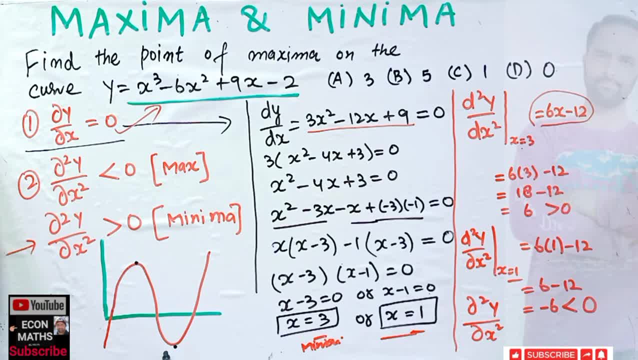 at this point we have, slope is equal to zero, and at this point we have: slope is equal to zero. okay, now to differentiate which of these two is maxima or minima, we use the second order condition. if the second order derivative is less than 0, we have a case of maxima, and here we can see that we 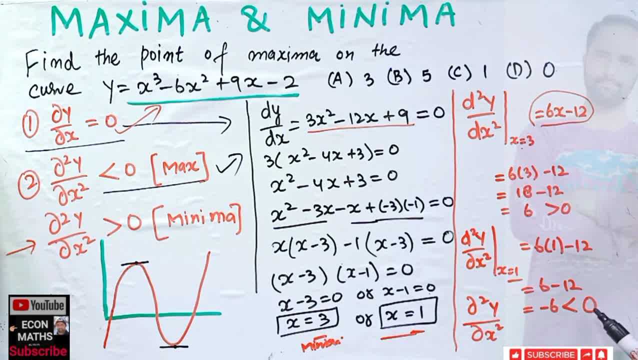 got second order derivative less than 0. okay, when X was equal to 1. that means at this point, if this is our X and this is our Y, so at X is equal to 1, our curve reaches at maxima and this point here, this point is actually, and this 3: okay. 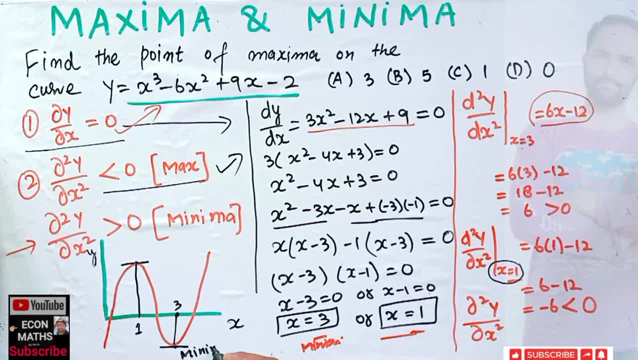 this is our minima and this is our maxima. okay, simple. first we said: first derivative equal to 0. okay, to get slope is equal to 0 and to check whether the second derivative is to see whether we have maxima or minima, we use the second. 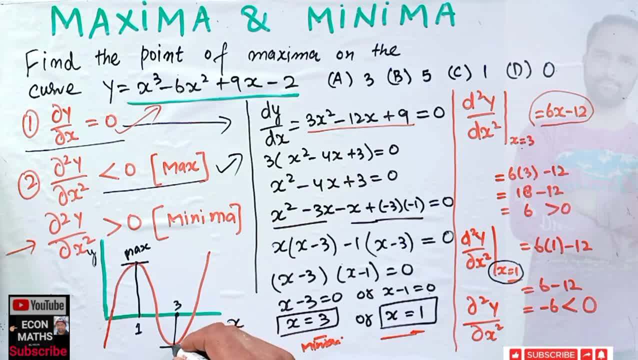 derivative- here we can see second derivative- is greater than 0. that means after reaching maxima and minima, if the slope increases, then we say we have a minima. similarly, if we reach here, the slope is equal to 0 and after that, if slope decreases, we have a case of maxima and